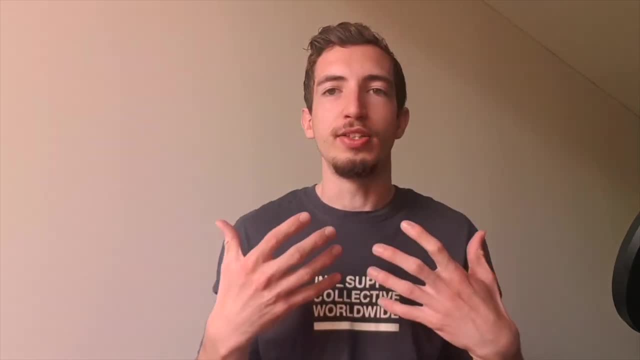 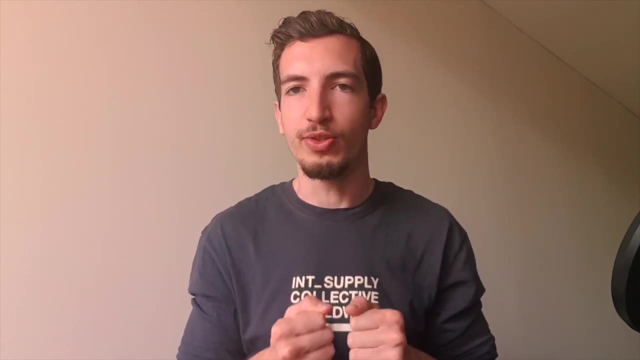 definition of deductive and inductive reasoning. and we're just going to get our hands dirty and look at some logical statements and trying to get into proofs as quickly as we can. So let's get into it. So let's now look at some basic notions from logic and 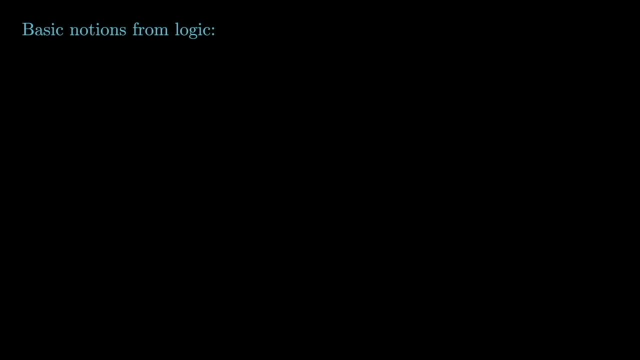 some basic definitions. These will help us to give a good framework for how to think about proofs and how to go about them. Let's define a proposition to be a statement which is either true or false. An example of a proposition could be that the earth is spherical. Another one could be that: 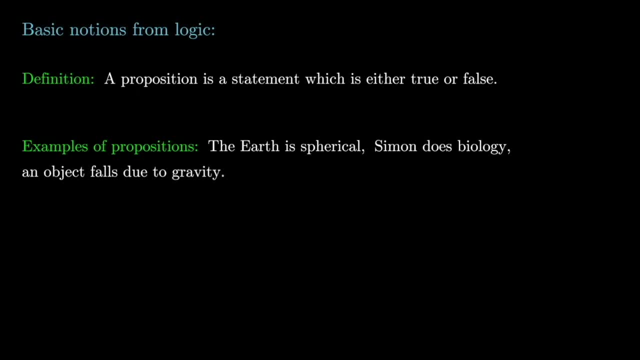 Simon does biology. Maybe one more would be that an object falls due to gravity. These statements are true or false. A premise will be a proposition from which another proposition is inferred, So it's a starting proposition from which we deduce a further proposition, And deductive reasoning is: 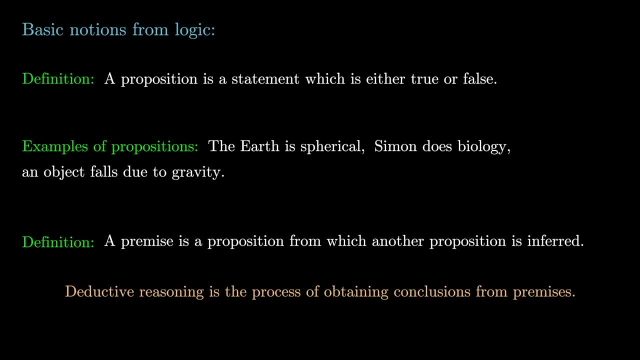 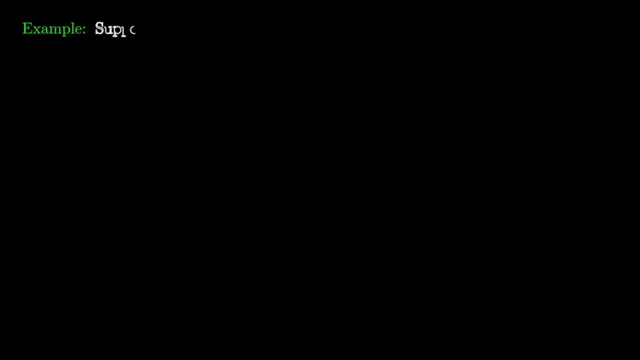 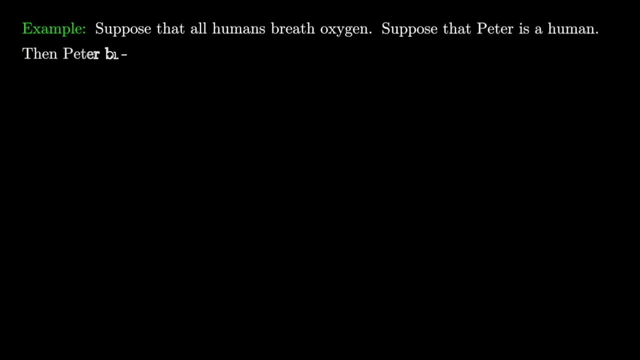 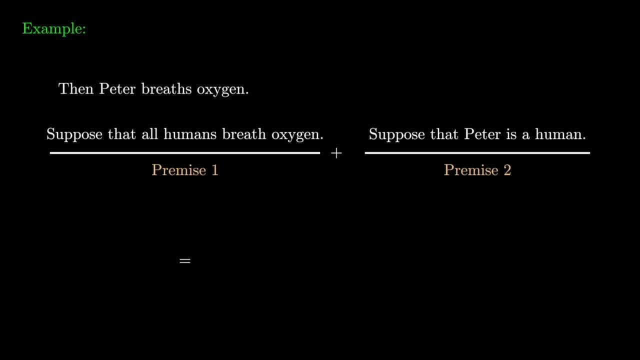 second premise And then the conclusion from which we got deductively was that Peter breathes oxygen. All that deductive reasoning is the process of obtaining conclusions from premises. We should emphasize that there's nothing here that requires the premises to be true. For example, 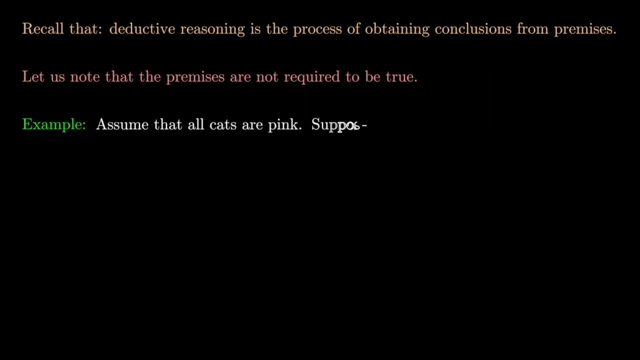 assume that all cats are pink And suppose Jamie is a cat, Then the true conclusion from these premises is that Jamie is pink. Maybe another interesting example is an example due to Bertrand Russell, which is suppose that 2 is equal to 1. And from this we can conclude that Bertrand Russell must be the pope. 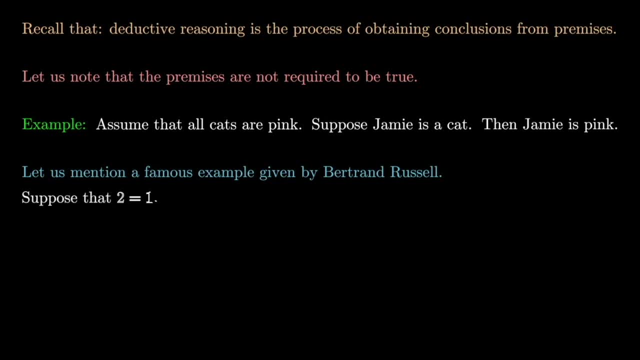 And from this we can conclude that Bertrand Russell must be the pope. The argument goes as follows: suppose 2 equals 1, well, we know that the Pope and Bertrand Russell consist of either two people or one person. Since 2 equals 1, however, it must be that Bertrand 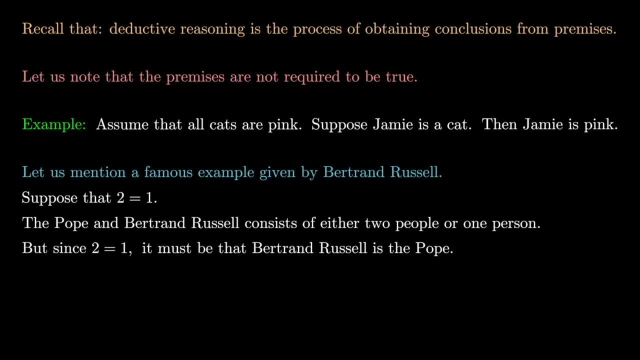 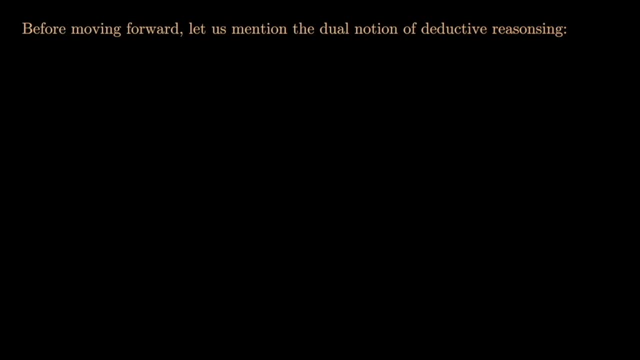 Russell is the Pope. Before moving forward, let us mention the dual notion of deductive reasoning, and this is inductive reasoning. Inductive reasoning is drawing inferences from true premises, so the conclusions from inductive arguments are less strong compared with the. 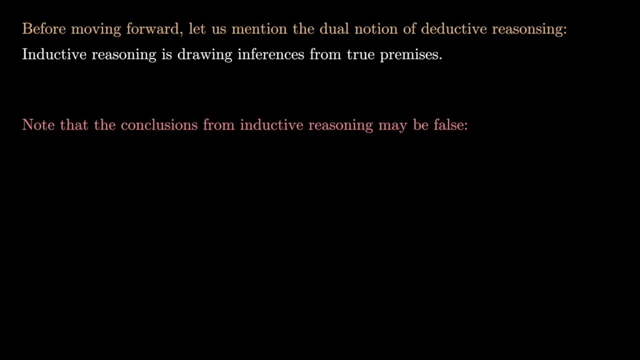 conclusions from deductive arguments. Here's an example of an inductive argument: the sun rises at 8am every morning. hence the sun will rise at 8am tomorrow morning. We're drawing an inference from a true premise, which may be wrong. it may not be the case that the sun rises at 8am tomorrow. 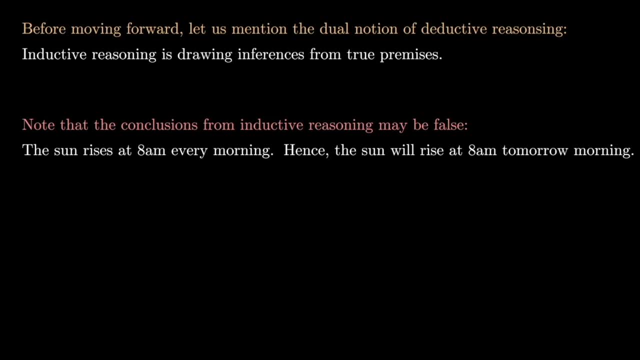 morning. For deductive reasoning, the premises are not required to be true, but the conclusion will be, While for inductive reasoning, the premises are always true, but the conclusions may be false. To test our understanding of deductive reasoning, let's take a look at 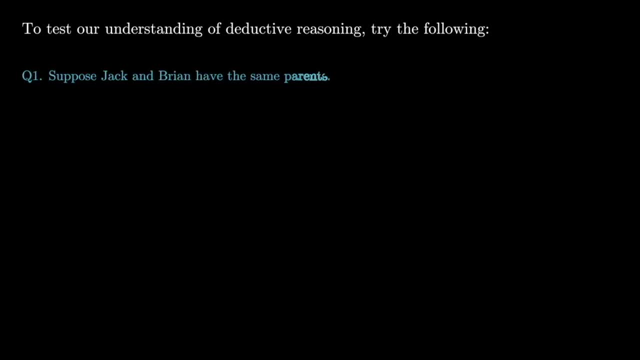 the following practice problems. Suppose that Jack and Brian have the same parents and assume that Jane has married Jack's brother. Are Jane and Brian married? Suppose the sum of two even numbers is odd. Prove that the sum of two odd numbers is also odd. 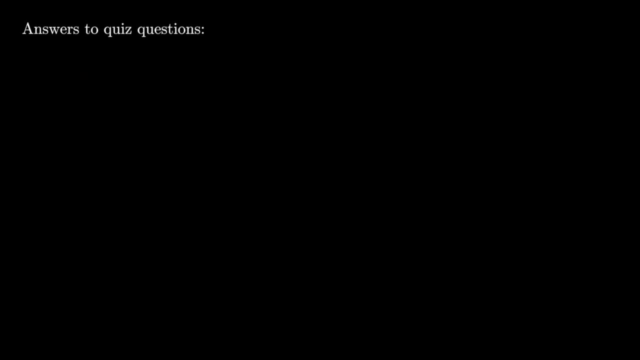 So let's look at the solutions to these quiz questions. Question 1, just to remind ourselves, was Suppose Jack and Brian have the same parents. Assume Jane married Jack's brother. Are Jane and Brian married? Of course we can't conclude that this is true, since Jack may have other brothers. 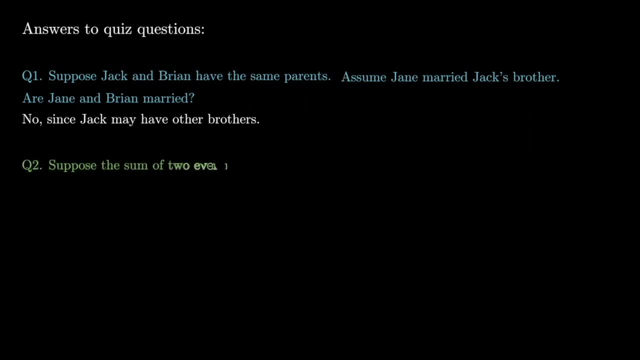 Okay, for the more interesting question. suppose the sum of two even numbers is odd. We need to deduce that the sum of two odd numbers is odd. Suppose that a and b are odd. then a can be written as 2m plus 1.